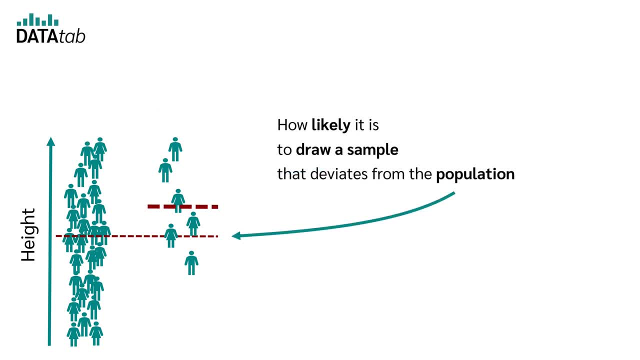 to draw a sample that deviates from the population by an equal or greater amount than the observed value. Let's take a closer look again. So we have a sample that is different from the population. We are now interested in how likely it is to draw a sample that deviates. 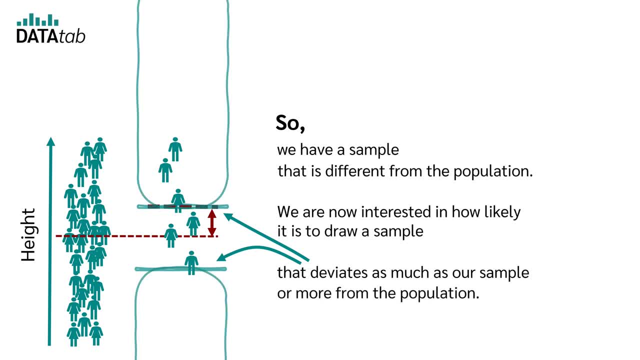 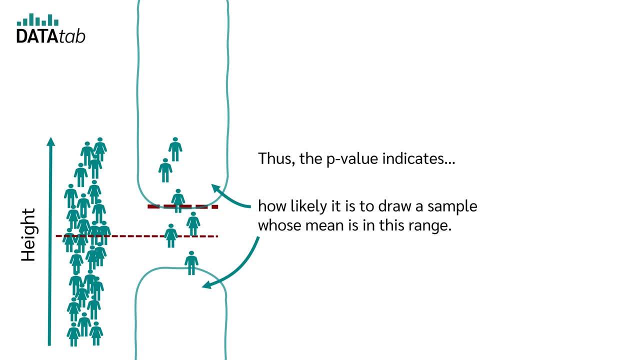 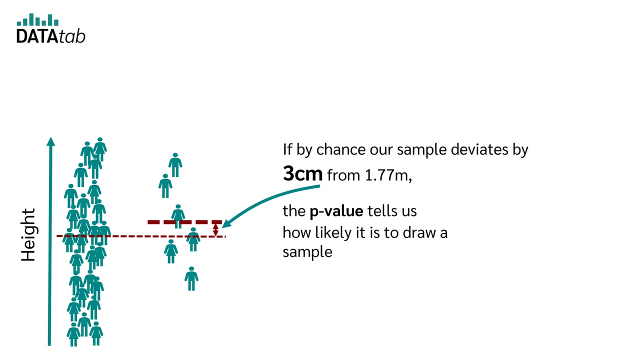 as much as our sample, or more, from the population. Thus, the p-value indicates how likely it is to draw a sample whose mean is in this range. If, by chance, our sample deviates by 3 cm from 1.77, the p-value tells us how likely it is. 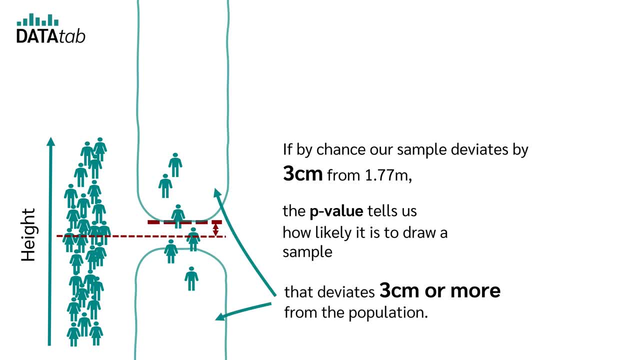 to draw a sample that deviates 3 cm or more from the population. If, by chance, our sample deviates by 1.77, the p-value tells us how likely it is to draw a sample that deviates 3 cm or more from the population. If, by chance, our sample deviates by 1.77,, the p-value tells us how likely it is to draw a sample that deviates 3 cm or more from the population. If, by chance, our sample deviates by 1.77, the p-value tells us how likely it is to draw a sample that deviates 3 cm or more from the population. 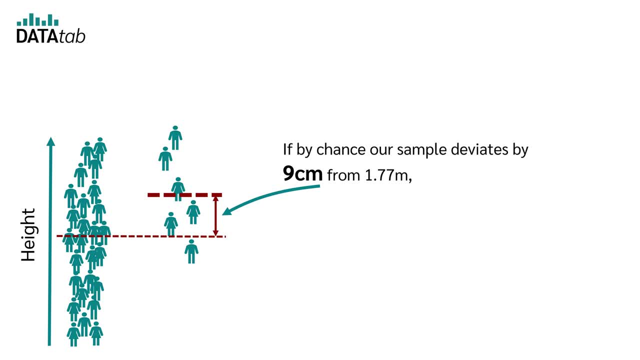 See now here our sample deviates by 9 cm from 1.77.. The p-value tells us how likely it is to draw a sample that deviates 9 cm or more from the population. Any example. So for our sample we get a difference of 9 cm. 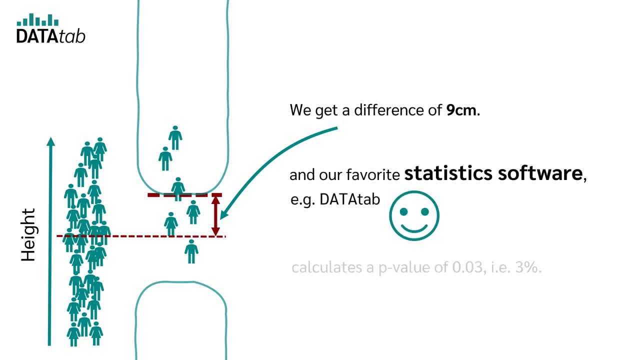 And our favorite statistics software, eg datatab, calculates a p-value of 0.03,, ie 3%. This now tells us that it is only 3% likely to draw a sample that is equal to or more than. 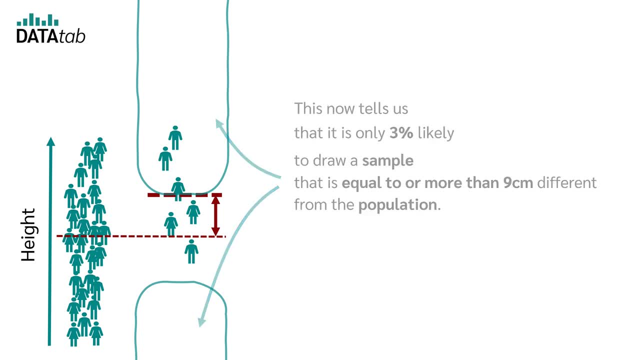 9 cm different from the population. For normally distributed data, this means the probability that the mean lies in this range is 1.5%. that the mean lies in this range is also 1.5% likely and together 3%. If this probability is very low, one can of course ask: 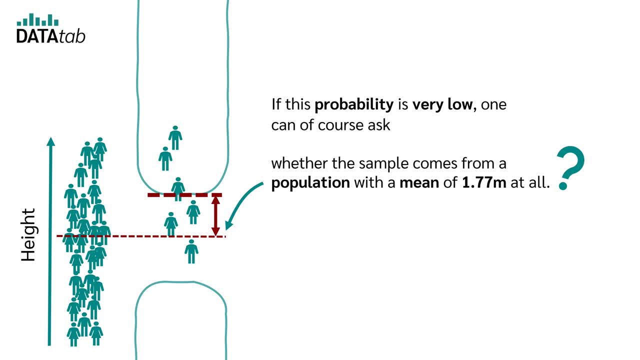 whether the sample comes from a population with a mean of 1.77 m at all. It is just a hypothesis that the mean value of basketball players is 1.77 m, and it is precisely this hypothesis that we want to test. Therefore, if we want to test the mean value of basketball players, we need to 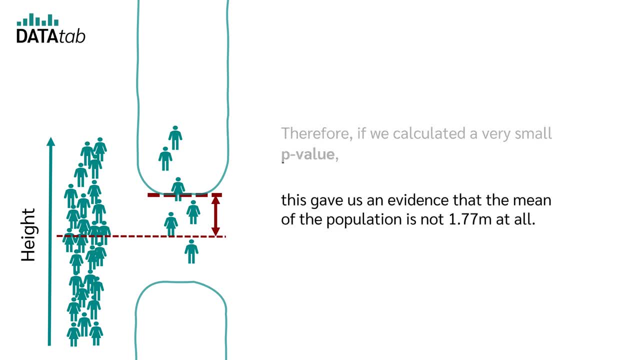 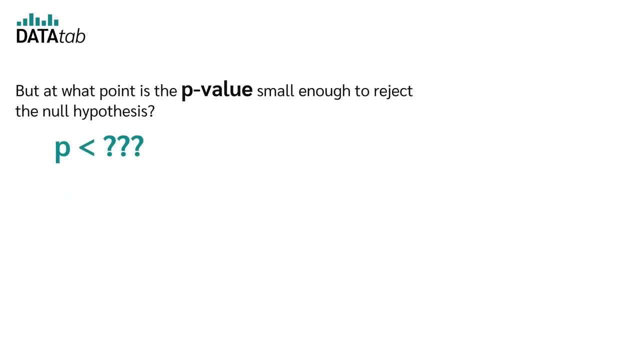 calculate a very small p-value. This gave us an evidence that the mean of the population is not 1.77 m at all. Thus we would reject the null hypothesis, which assumes that the mean is 1.77 m. But at what point is the p-value small enough to reject the null hypothesis? 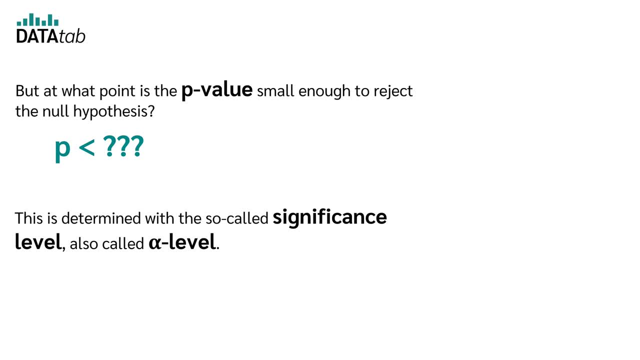 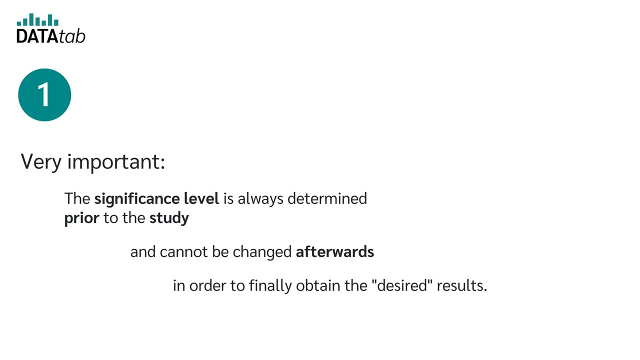 This is determined with the so-called significance level, also called alpha level. There are two things to notice here. 1. Very important: The significance level is always determined prior to the study and cannot be changed afterwards in order to finally obtain the desired results. 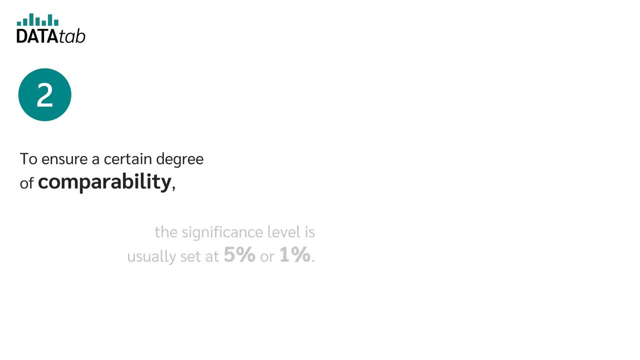 2. To ensure a certain degree of comparability, the significance level is usually set at 5% or 1%. A p-value of less than 1% is considered highly significant, Less than 5% is called significant and greater than 5% is called not significant. 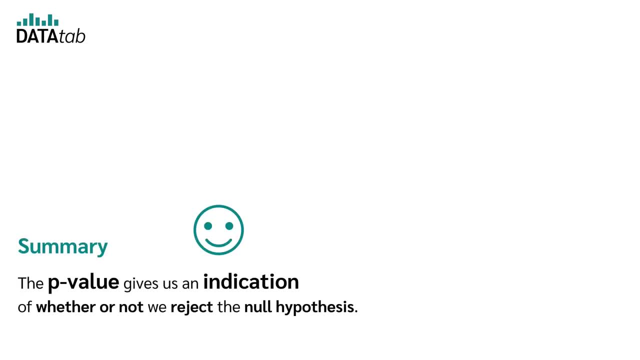 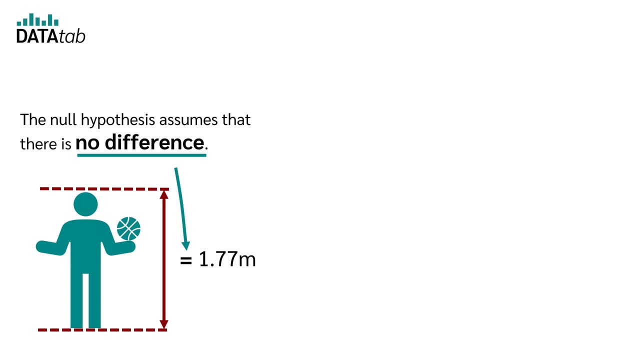 Summary: The p-value gives us an indication of whether or not we reject the null hypothesis. As a reminder, the null hypothesis assumes that there is no difference. In contrast, the alternative hypothesis assumes that there is a difference. In general, the null hypothesis is. 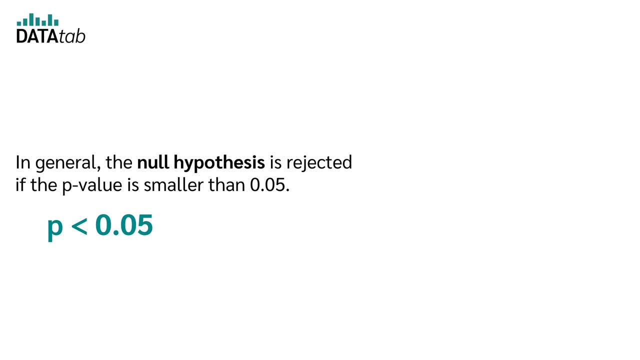 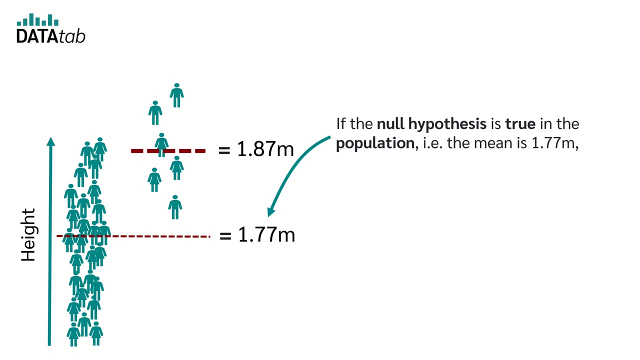 rejected if the p-value gives us an indication that the null hypothesis is rejected is smaller than 0.05.. However, as we know, it is always only a probability and we can be wrong with our statement. If the null hypothesis is true in the population, ie the mean is 1.77 meters. 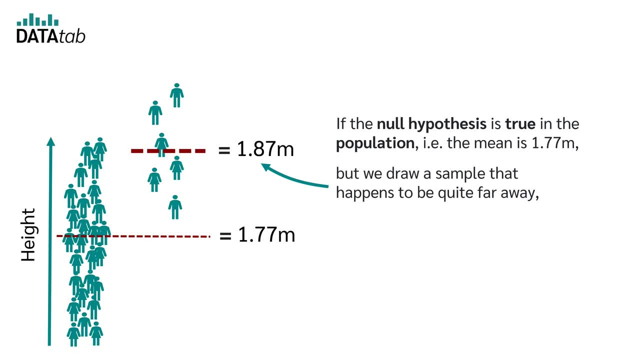 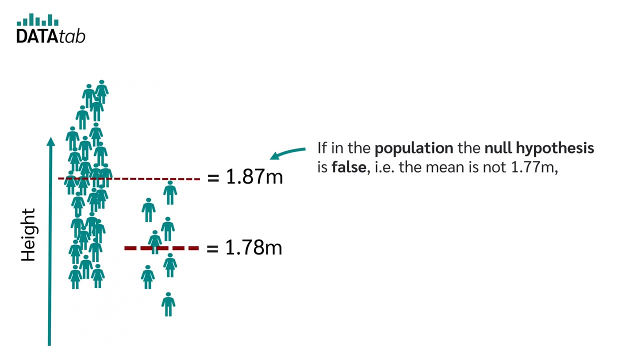 but we draw a sample that happens to be quite far away. it might be that the p-value is smaller than 0.05, so that we wrongly reject the null hypothesis. This is called type 1 error. If in a population the null hypothesis is false, ie the mean is not 1.77 meters. but we draw a sample. 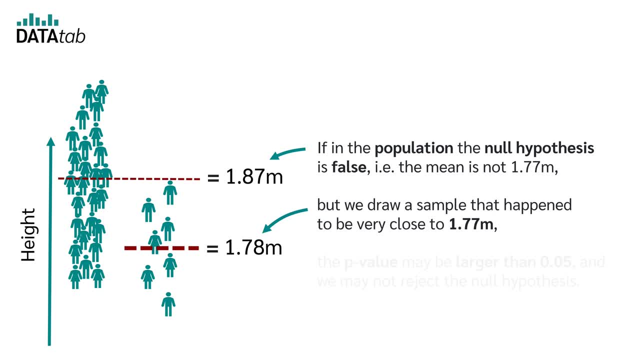 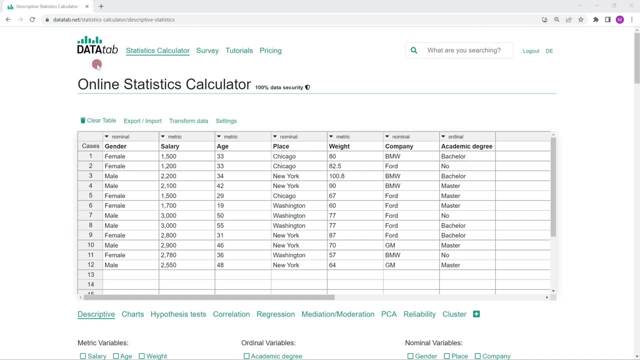 that happens to be very close to 1.77 meters. the p-value may be larger than 0.05, and we may not reject the null hypothesis. This is called 0.05.. Type 2 error. And now I will show you how you can easily calculate the p-value for a variety of hypothesis. 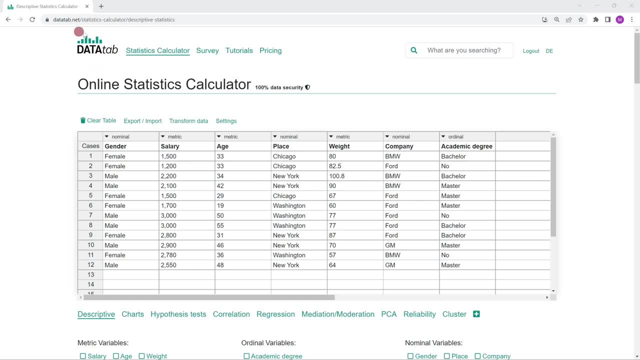 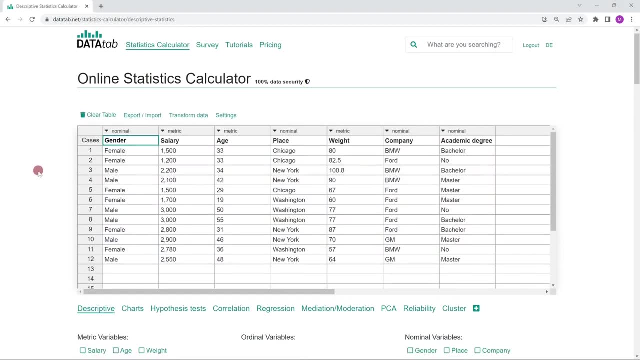 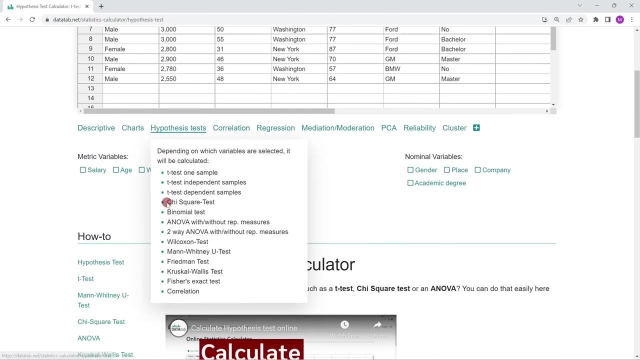 tests online with DataTab. To do this, simply visit data-tabnet, copy your own data into this table and click on Hypothesis test. Depending on which variables you click on, DataTab will suggest a hypothesis test, For example, a t-test, chi-squared, etc. 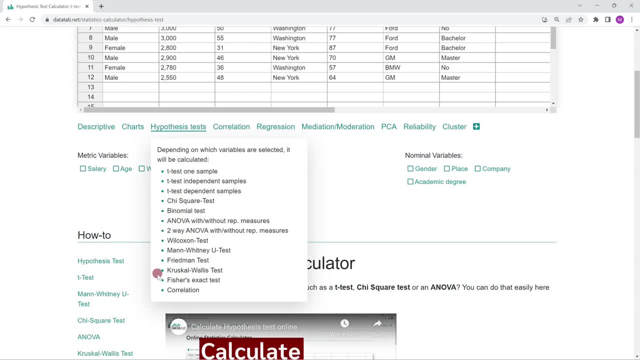 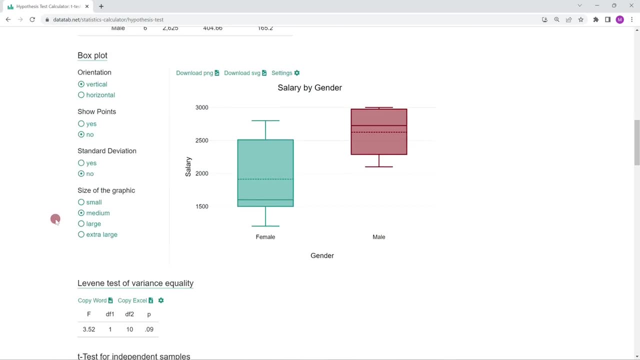 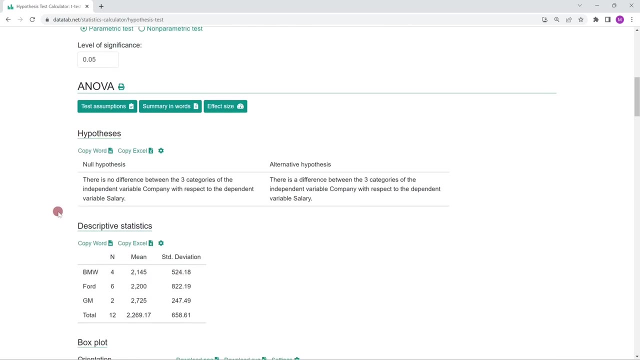 A square test, ANOVA, Wilcoxon test and many more. For example, if you click on Celery and gender, a t-test for independent samples is automatically calculated. If you click on Celery and company, for example, an analysis of variance is automatically calculated. 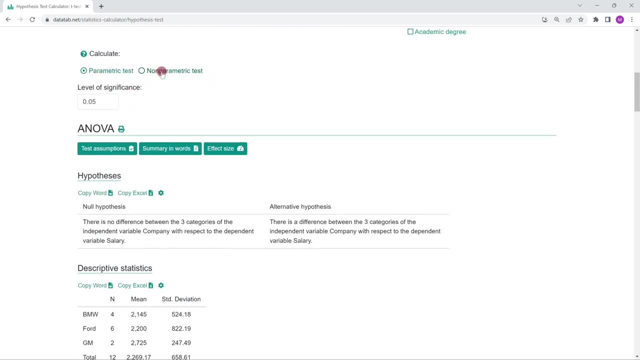 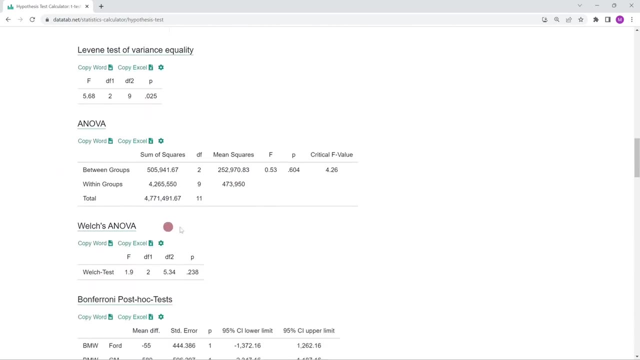 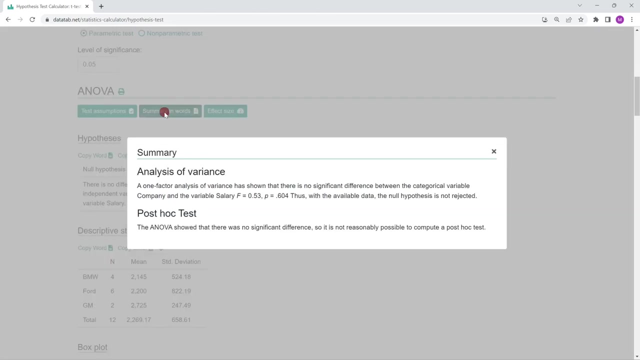 If your data is not normally distributed, you can also calculate the non-parametric counterpart. If you now scroll down, you will find the p-value. If you are not sure about the interpretation, you can click on Interpretation in words. A one-factor analysis of variance has shown that there is no difference. 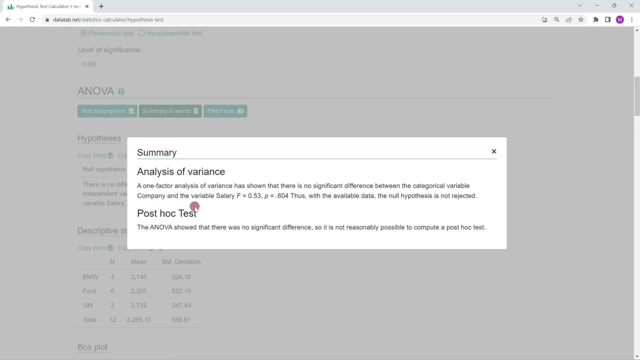 between the categorical variable company and the variable Celery. Thus, with the available data, the null hypothesis is not rejected. Thanks for watching. I hope to see you soon. 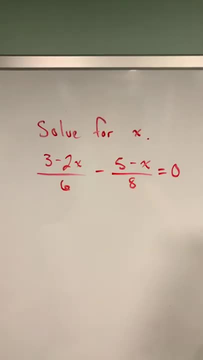 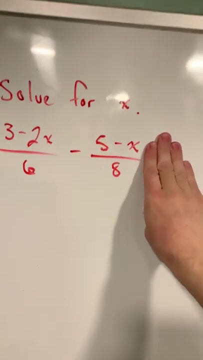 Let's solve for x in this rational equation. Now, the first thing I would do is I would take this expression here and move it over to the right side, and I would do that by adding: but since I'm working on a whiteboard, I'm going to just going to go ahead and yoink. So you can. 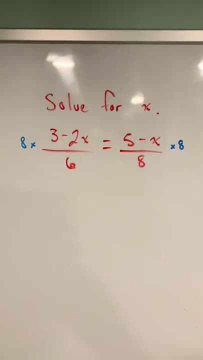 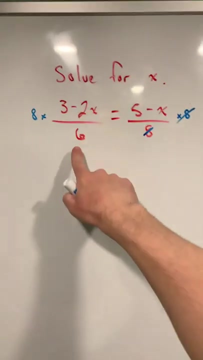 imagine that I just took that expression and moved it over to the right side of the equation. To clear out these fractions, I'm going to multiply both sides by 8, which is going to get rid of my denominator of 8 on the right hand side, and I'm going to do the same thing with the 6 on the left. 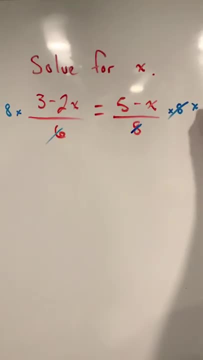 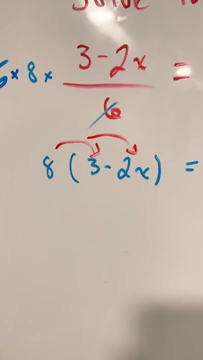 hand side. Multiplying by 6 allows me to cancel them out, but I also have to do that on the right hand side. So if we clean this up a little bit, we're left with an equation like this: I can use the distributive property on the left hand side to multiply the 8 into the brackets, and I can do. 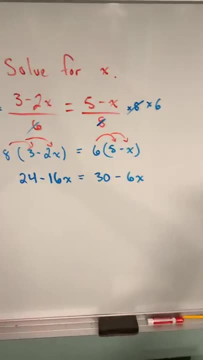 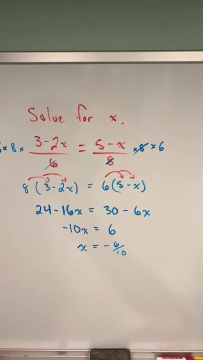 the same thing on the right hand side. We end up with a pretty simple linear equation with an x on each side. We'll apply some basic algebra to move the x's to the left side and the non-x terms to the right side. Dividing both sides by negative 10 results in x equals negative 6 over 10. also.